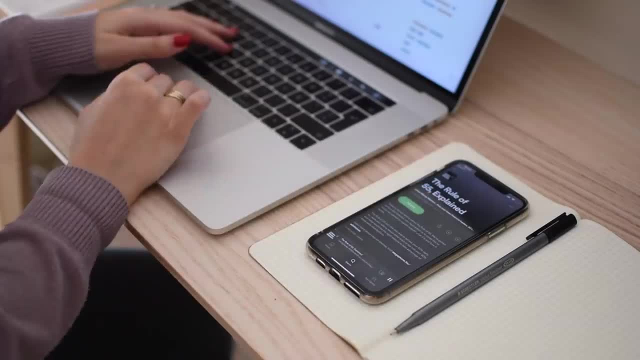 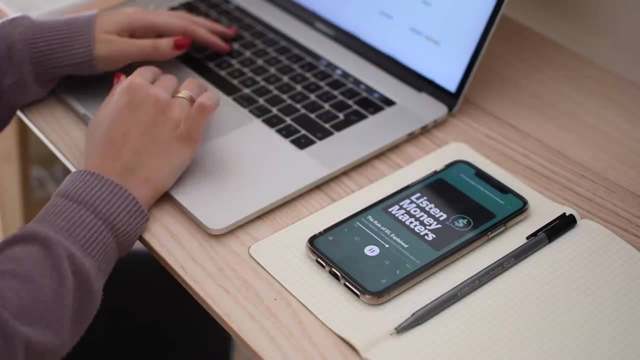 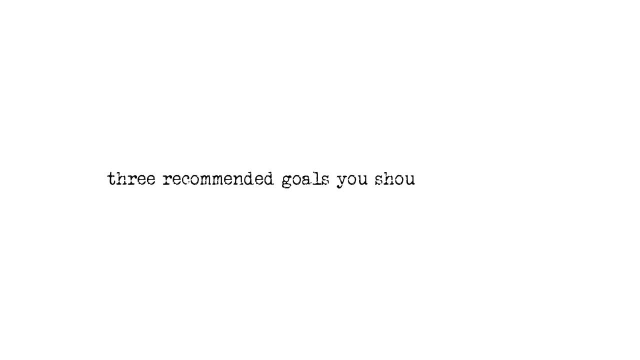 can be done in a very guilt-free environment. Everyone makes mistakes and may let things slip by. If you are in that situation, you're not alone and we're all in the learning process together. Okay, so usually if you're starting out with personal finance, there are three recommended. 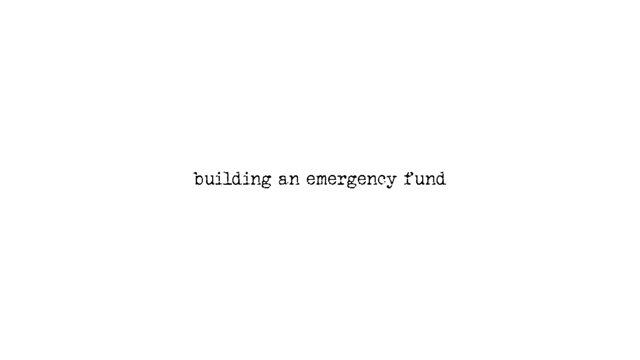 goals you should prioritize: Building an emergency fund, starting budgeting and tracking your expenses, and getting rid of debt. Regarding this last point, I will link down below some useful resources, videos and articles for more in-depth analysis. Let's start talking about the emergency fund. A full emergency fund should vary between three to six months of expenses. You need your emergency fund because life is unpredictable and there are sometimes incredibly large and unforeseen expenses that may throw you off-balance. For many specialists on personal finance, the emergency fund should be your first goal. 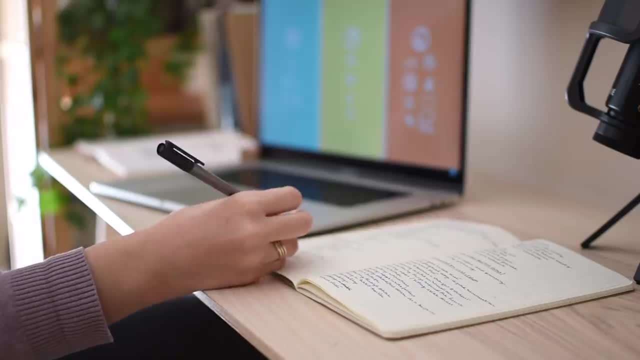 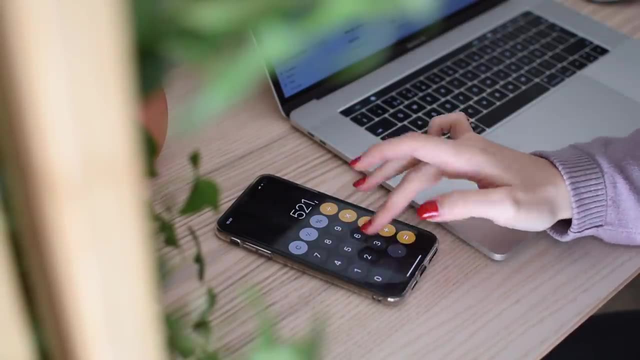 if you're started on this path. Also, you should always have your emergency fund fully stocked. That means that if, for some reason, you need to use your fund, all of your saving priorities for other secondary goals should be dropped to restock the emergency fund again. 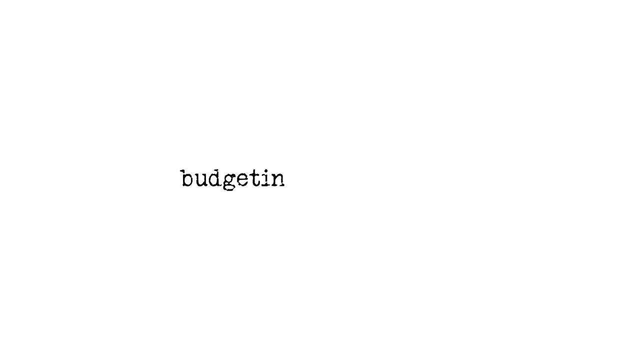 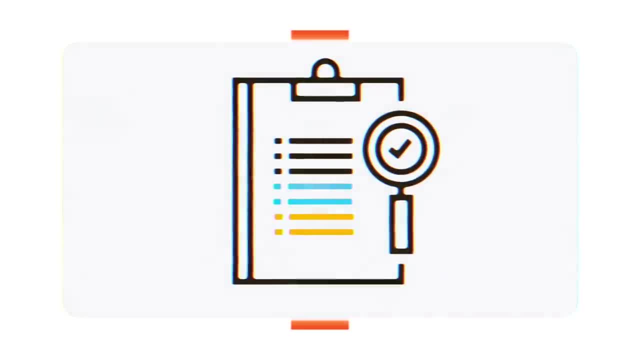 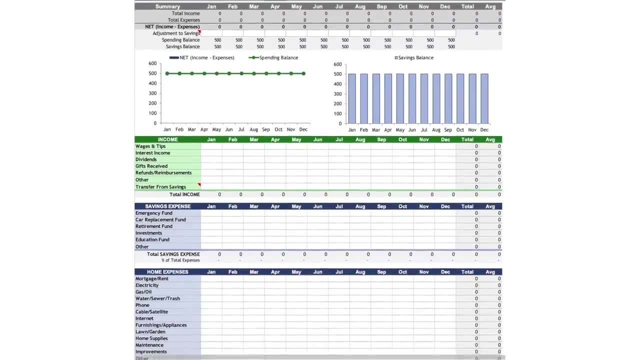 money. There is a lot to say about this. Budgeting and tracking more-than-specific goals you need to achieve are habits you should start strengthening and implementing early on. If you're feeling a bit lost as to where your money is going, I highly suggest you. 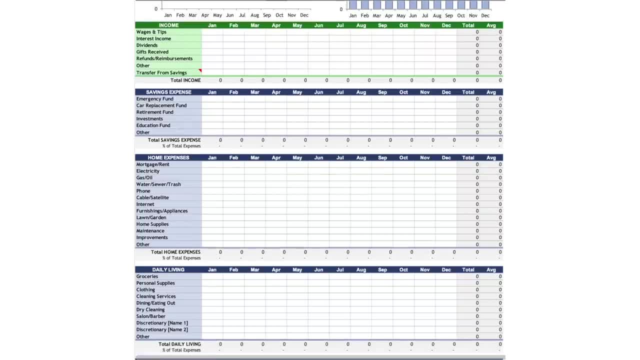 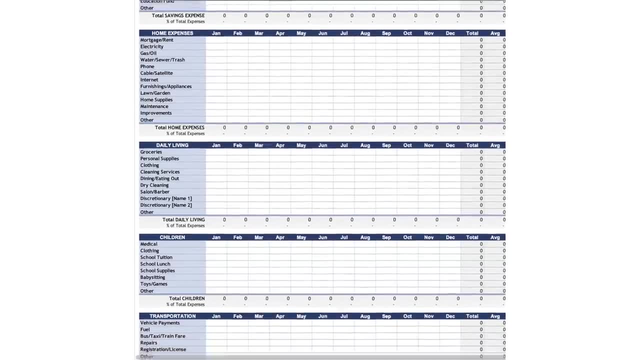 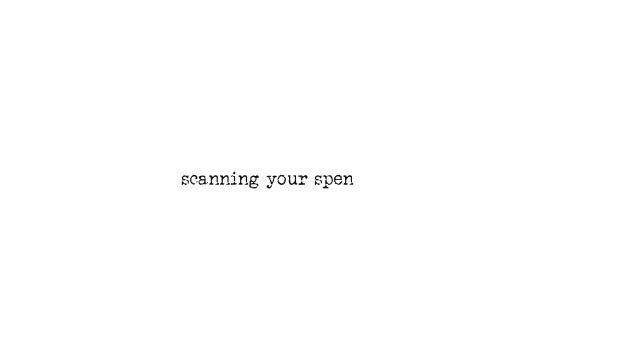 to regularly track your expenses. This may seem completely useless at first, since you're probably just either copying your expenses from your banking extract or manually filling in where you spend your pocket money. scanning your spending habits, You'll find out how regularly you're spending money and where you're able to cut or not. 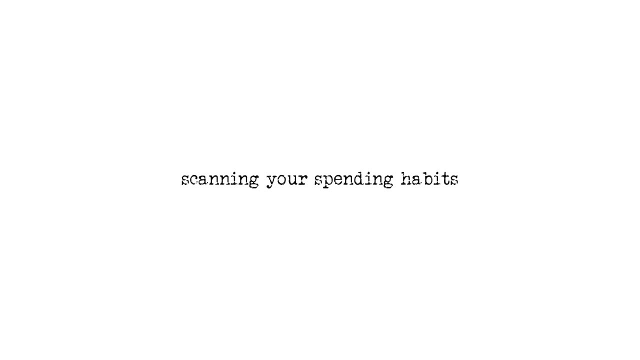 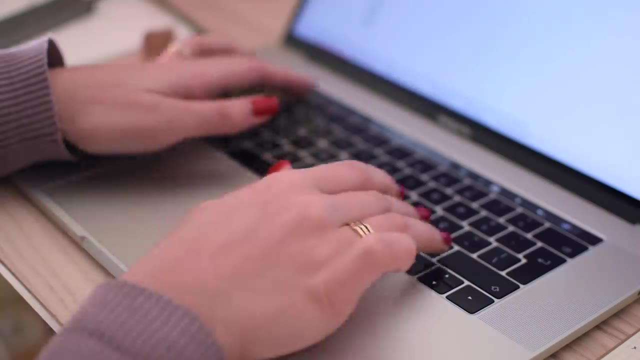 Believe me, most of you will get a heck of a surprise when you start doing this. Implementing the habit of just tracking your expenses on a simple Excel or Google spreadsheet every single day is a good way to make sure you're doing this without the overwhelming 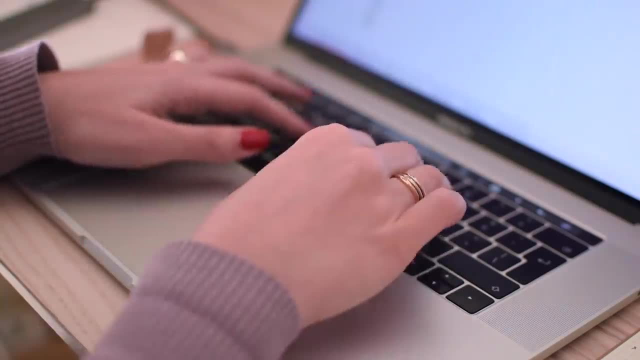 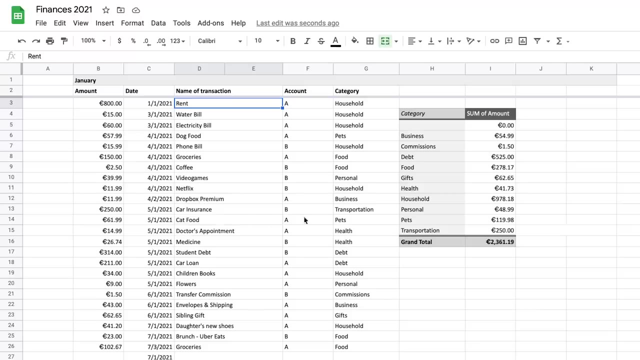 task of having to do it on a monthly or weekly basis, Because those numbers pile up pretty fast. Personally, I track my expenses daily and I use Google spreadsheets simply because I can access it anywhere without worrying about the integrity of the file. 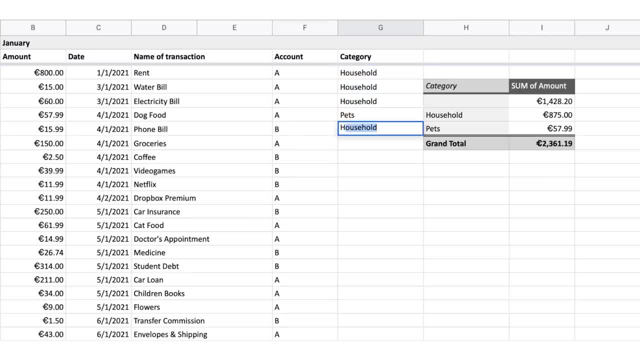 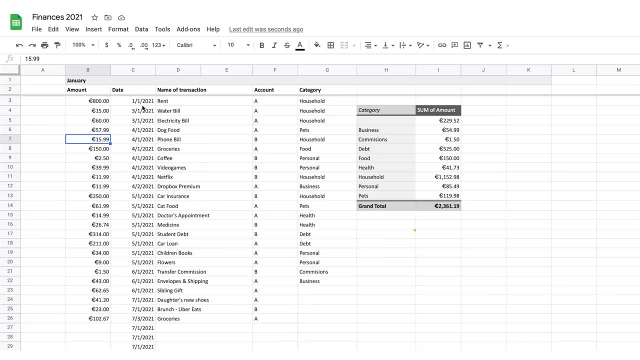 Regarding expense tracking, don't settle only on listing expenses. Going one step further in terms of your analysis of your financial situation can really make a difference in the end. For instance, make sure you're categorizing your expenses so you can really dig in and 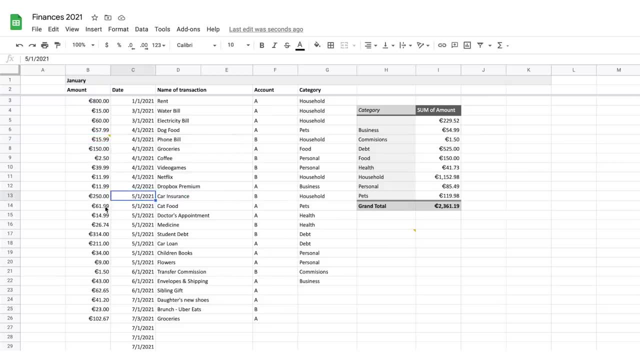 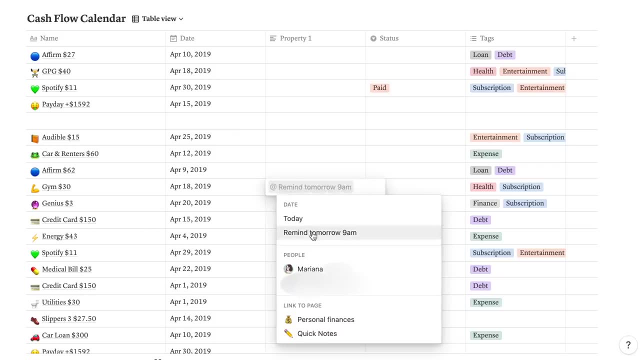 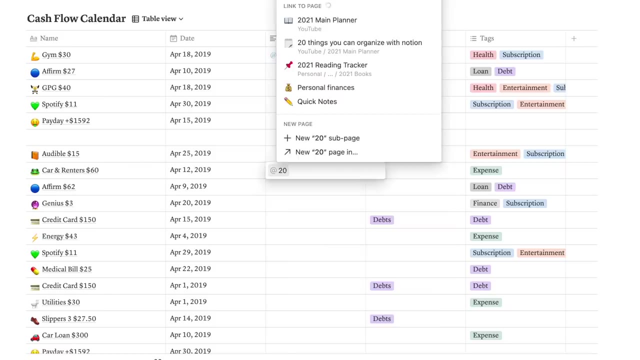 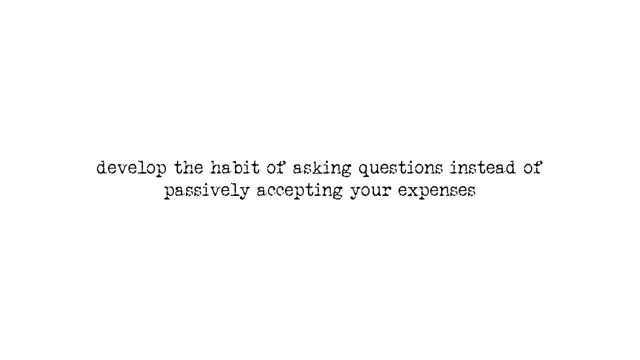 see which categories are representing the biggest slice of your budget. Add comments and set reminders. signal which expenses were unnecessary and which you want to avoid in the future, and signal which expenses represent something you may either reduce or eliminate altogether. Also, take this time to develop the habit of asking questions instead of passively accepting. 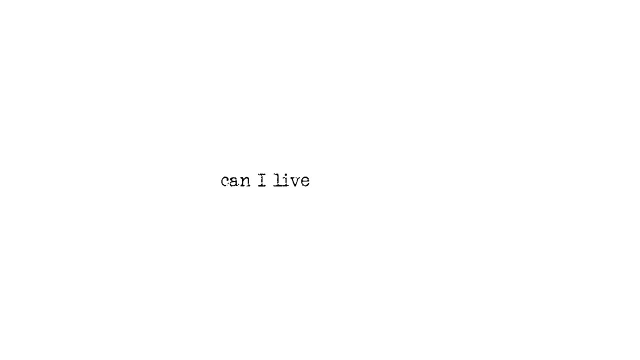 your expenses. Ask things like: can I live without it? Can I live without it? Do I need it? Can I afford it? Can I lower or cut back on this expense? These questions will help you reduce your expenses, bit by bit. 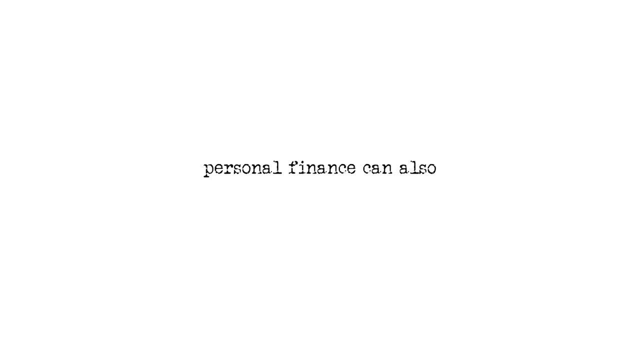 Much like other areas of your life, personal finance can also be a mindful process that helps you prioritize in terms of money management, in this case, what you prioritize in life and what you should cut back on. There are some interesting budgeting rules of thumb. 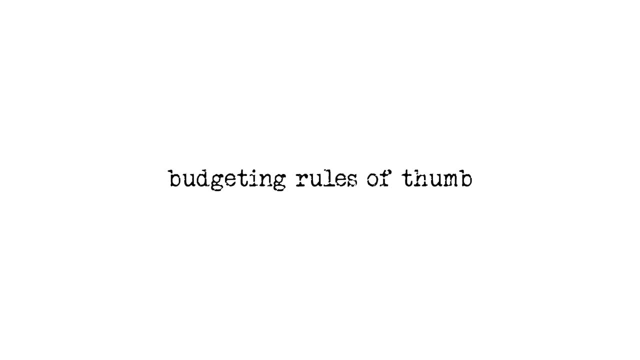 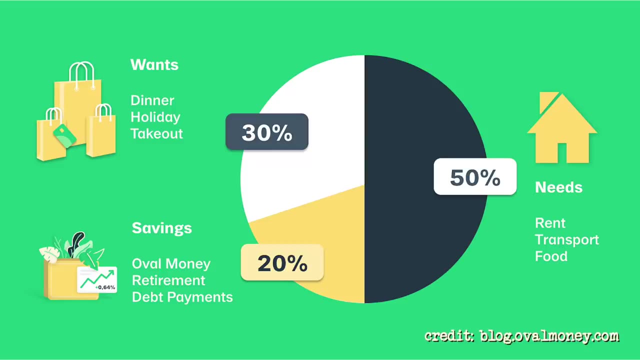 Or even you can experiment with or even implement in case it makes sense for you and your situation. The 50-30-20 rule is a general budgeting rule that's very famous and it states you should spend 50% of your income for Necessities like housing and bills, 30% for Wands and 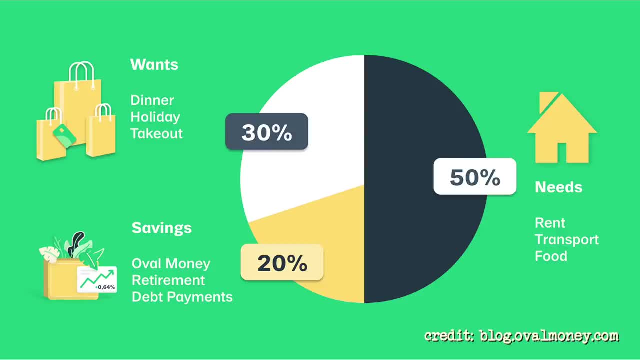 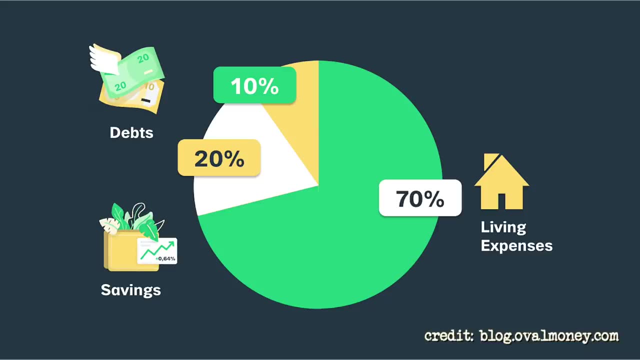 personal purchases and 20% for financial goals like paying off debt or saving for retirement 8.. Another variation of this is the 70-20-10 rule, which recommends you save 70% for your living expenses, 20% for savings of your net salary and 10% for debt payments. 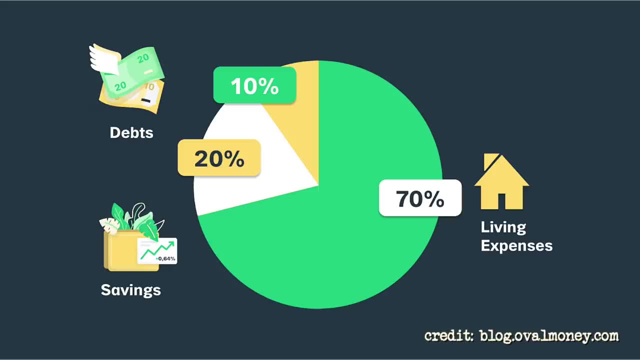 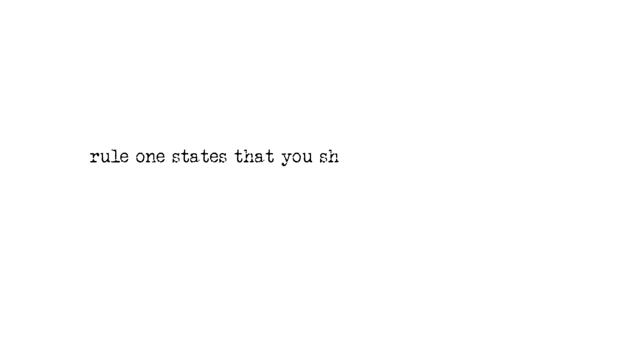 In this case, the recommendation is to pay off the most damaging debt first and then focus on paying off the rest as quickly as possible. Rule 1 states that you should prioritize how you'll use your money and how independently of how much you earn. 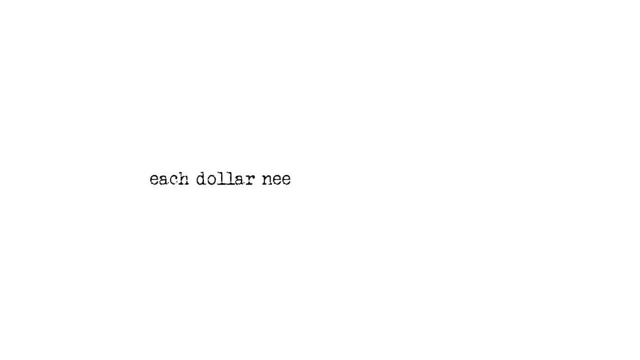 As soon as you get your money, you need to decide what to do with it. Each dollar needs to be assigned a job, And then you just have to follow your plan. For instance, if, after paying your bills, debt and other necessary expenses, you still 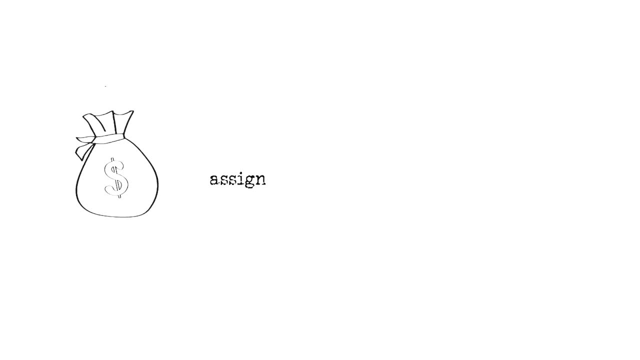 have $100 remaining in your account. assign each one of those dollars a task. For instance, you may decide that you want to spend no more than $50 dining out that month, $20 on new books and $30 on new fitness equipment. 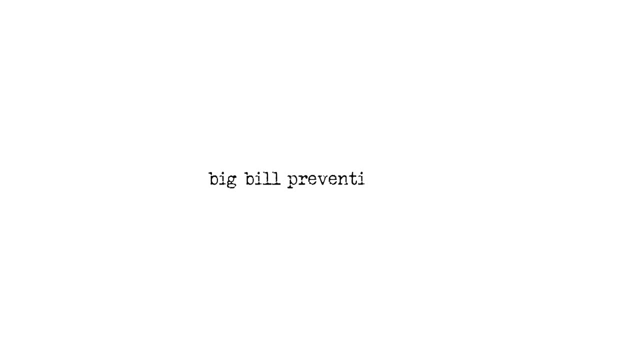 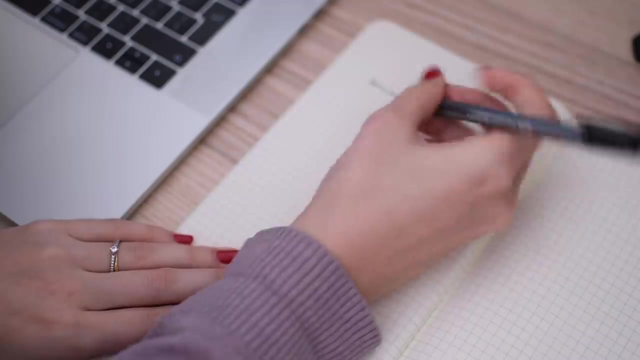 Rule 2. Big bill prevention rule is used to avoid big payments like an annual car repair or revision, Christmas or birthday gifts, an annual weekend out, etc. Once a year. sum all of those expenses the money you want to allocate for gifts regular. car or house repair expenses and divide it by the 12 months of the year. Your goal is to fund those extraordinary expenses monthly And when the bills arrive you already have the money and will be able to avoid extra debt or expenses. And finally, the 20-4-10 car loan rule helps clarify how you should allocate your money. 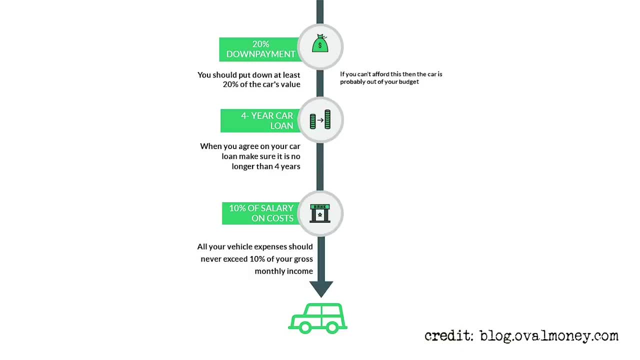 towards purchasing a car and how Basically it states you should make a 20% down payment that will keep you from owing more than your car is worth. with the loan under 4 years, This will help you minimize the amount of interest you pay over the lifetime of your 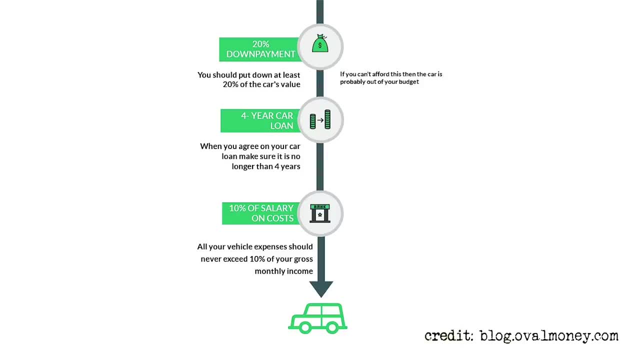 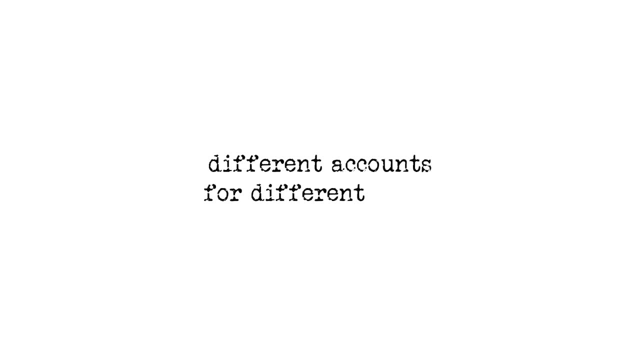 loan And, finally, your car payment should be kept under 10% of your gross monthly income. If you currently have a specific financial goal in mind, you may consider creating accounts for different goals. This, of course, depends on where you live, as well as the rules in your country. 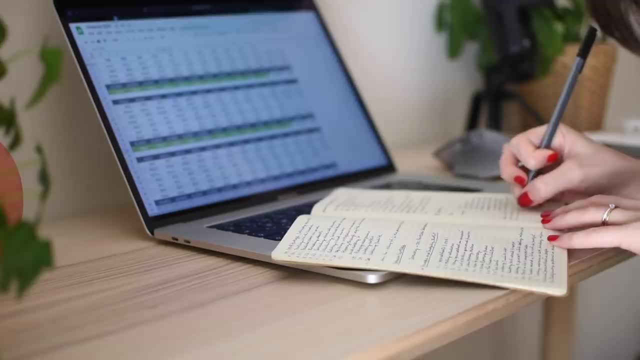 But there are cases in which you can create an account without having to pay regular commissions. In that situation, it may be a good idea to create your own account. If you have a specific financial goal in mind, you may consider creating accounts for different. 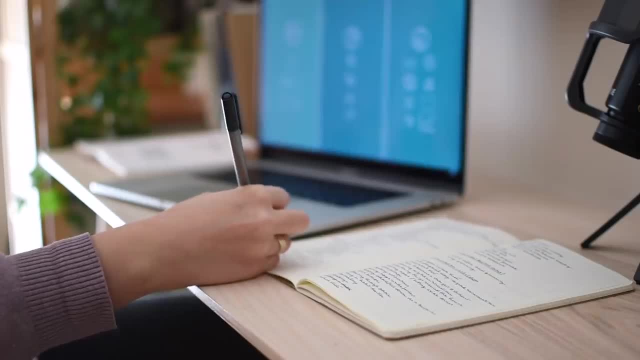 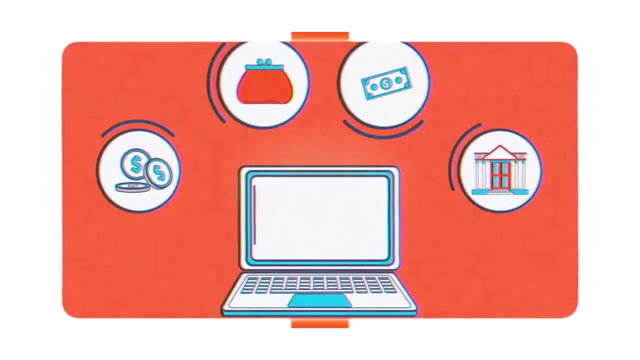 goals. You may even consider creating a new account for that goal and set up automatic transfers. Each time you get your paycheck, a specific amount will go to that account and you know that money is untouchable. When me and my fiancé were saving for our wedding, this is exactly what we did. 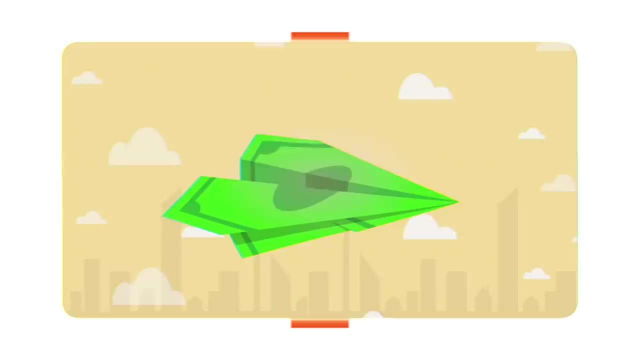 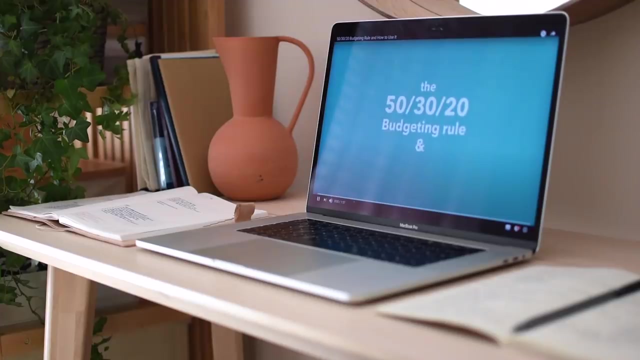 We created a new bank account. we set up a monthly automatic transfer and never asked for any kind of credit or debit card associated with that account. We used that money to save our wedding. This is exactly what we did. We created a new bank account. 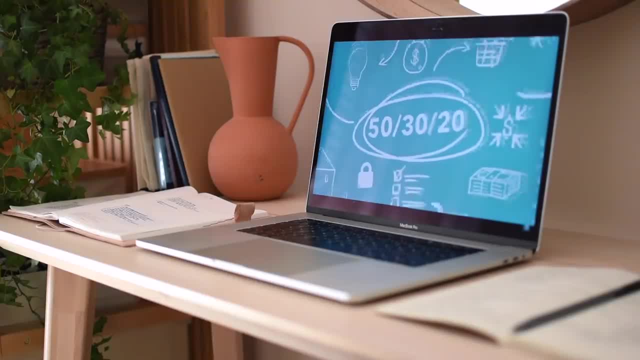 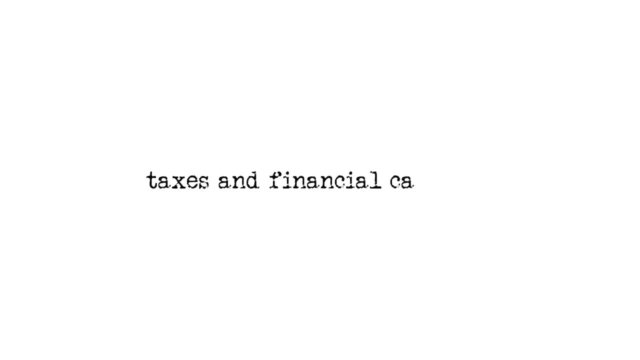 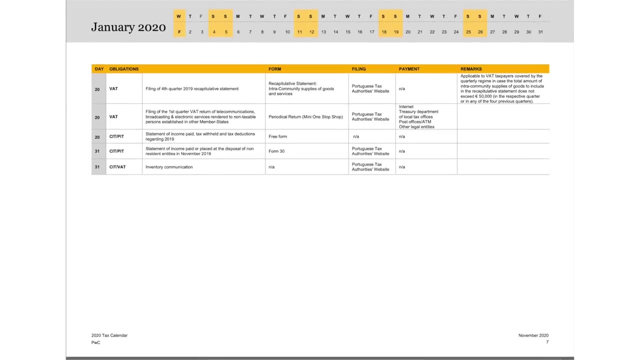 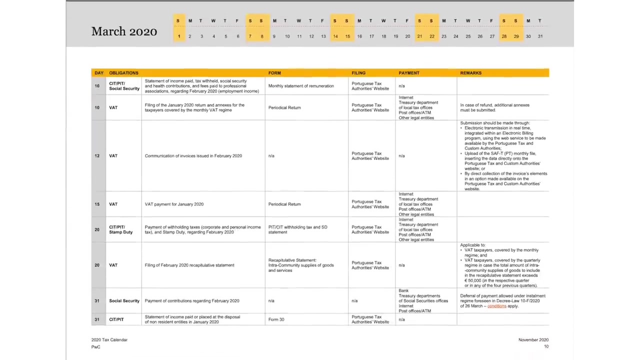 reachable for regular expenses, unless I was transferring the money over to pay the vendors, the catering, etc. Unfortunately, personal finance is not all about saving and tracking and reducing expenses. Planning correctly for your taxes is also essential. Once again, this completely depends on where you live, but you can probably find a tax. 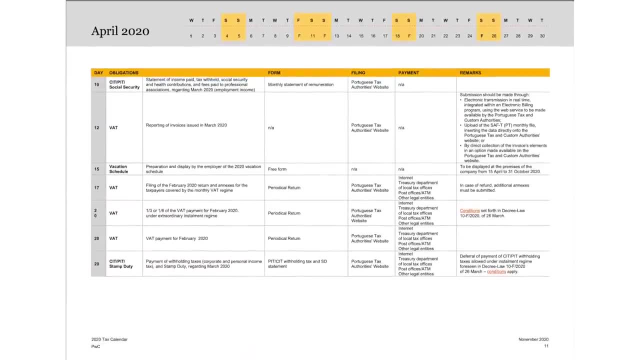 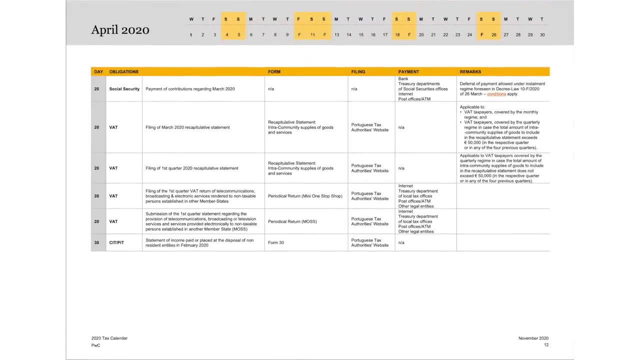 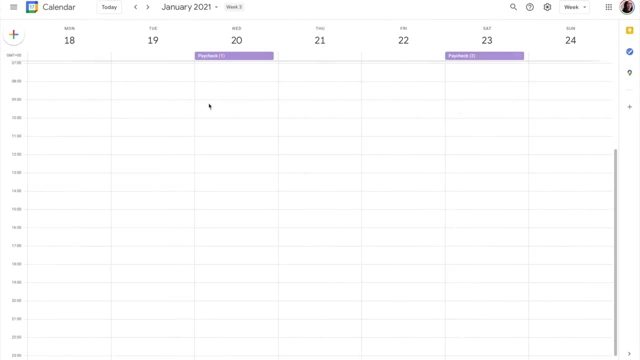 calendar available on the internet for your country. Besides organizing your expenses, taking into account your tax bill, you should also make sure you're organizing and tracking the receipts that you can offset against that tax bill, Also scheduling your bills are due. You can use all different types of software for this, as well as a paper planner. 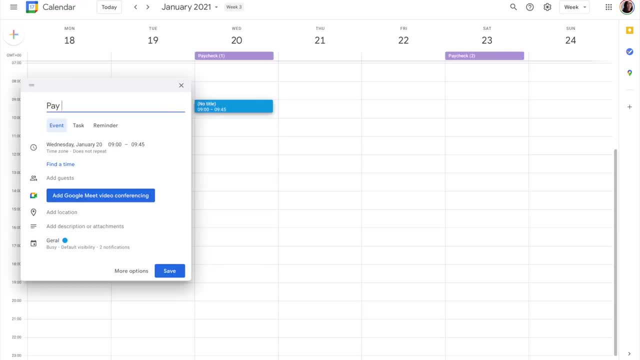 If you can try to pay all of your bills on the same day of the month. For instance, if you have 10 bills to pay and they spread out across your monthly calendar – schedule to pay the 10 bills on the due date of your first one. 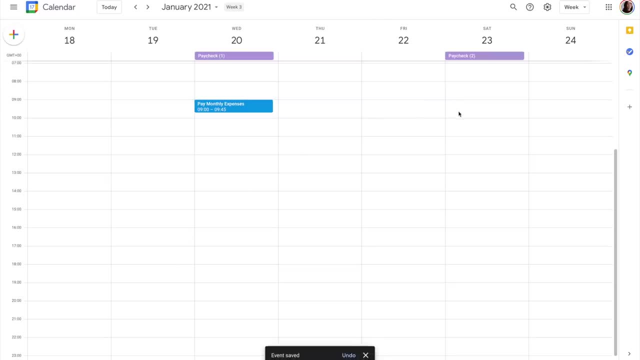 Even if you're anticipating your payments, you're paying everything in time and you will avoid thinking about it for an entire month. Also, the advantage of paying all of your bills on the same day and making your saving transfers on that day as well ensures that whatever is left on your account is for your personal. 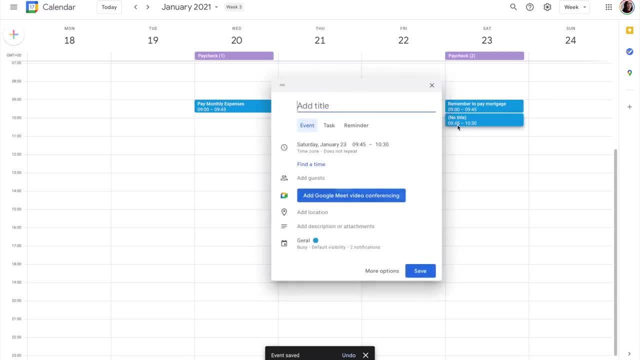 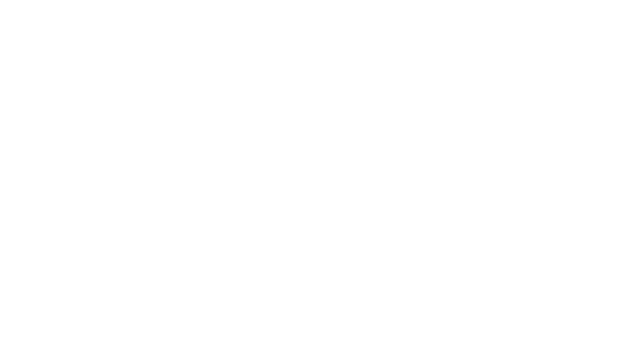 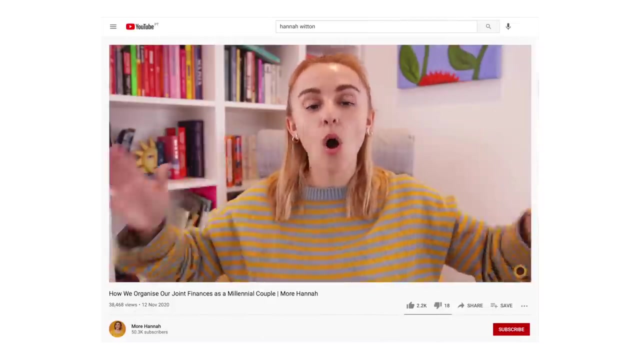 spending, making it much easier to manage until the end of the month. Finally, implement the habit of regular finance housekeeping. Consider that managing your expenses and the expenses of your family is a chore. The first person I heard mention this was Hannah Witton, and I think she's absolutely. 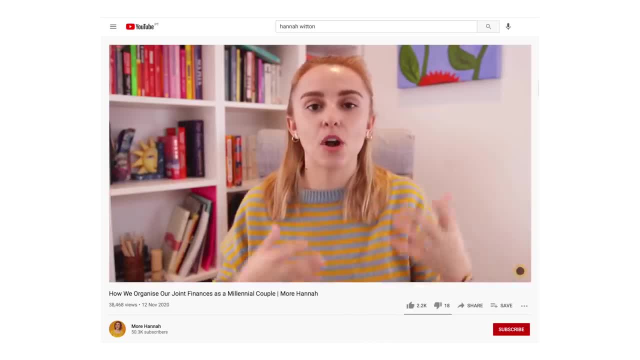 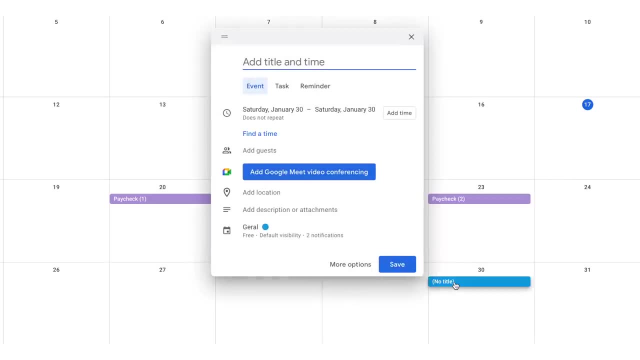 right. Tracking, budgeting and remembering when to pay the bills may be something that only one person may have in mind, and it's basically a chore like any other. That change of mindset may allow you to regain some control of your personal finances. 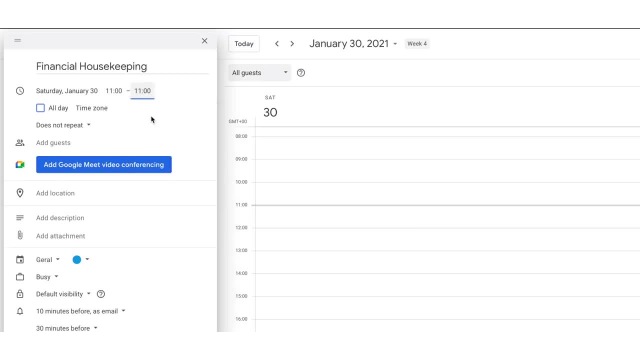 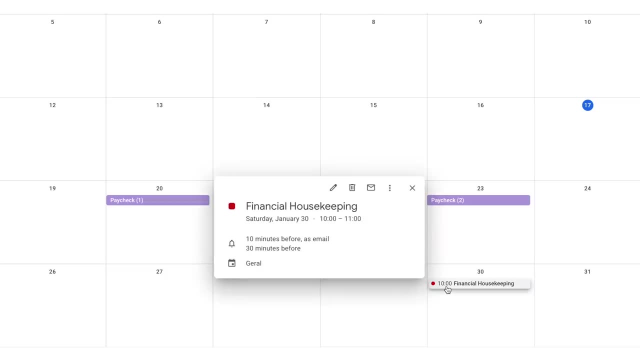 Schedule in your planner these financial housekeeping sessions, check your accounts and ensure payments are arriving, file receipts, check that you're paying your bills and schedule any other payments in advance. I will also link down below an empty template of my current expense and budget tracking. 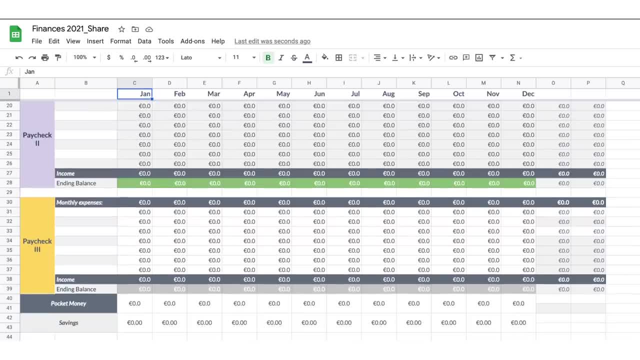 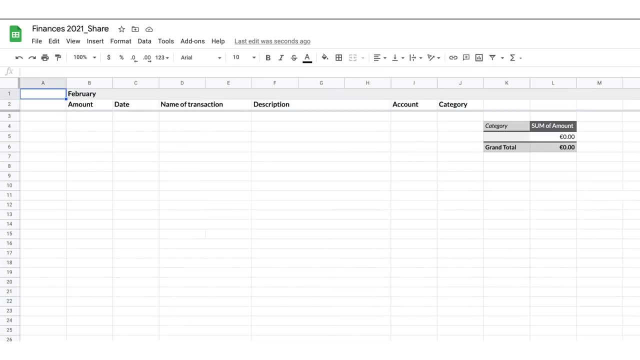 spreadsheet in case you don't want to build it from scratch, And I will also link down below a couple of Notion templates with expense trackers and other personal finance templates, in case you prefer that method, Although I'm a huge believer that you can start learning new things and developing. 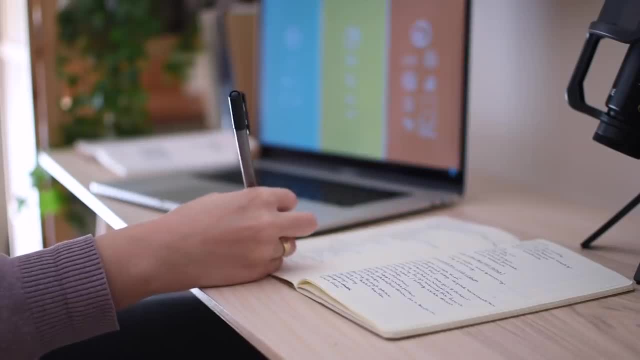 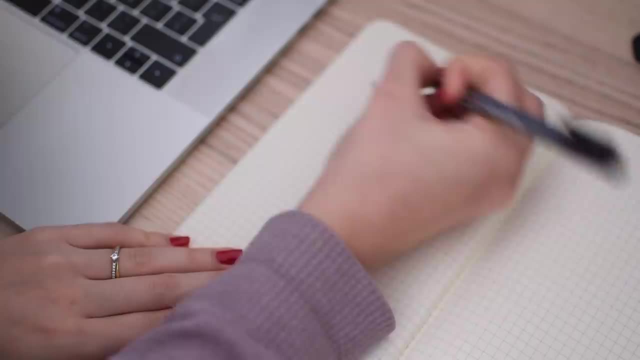 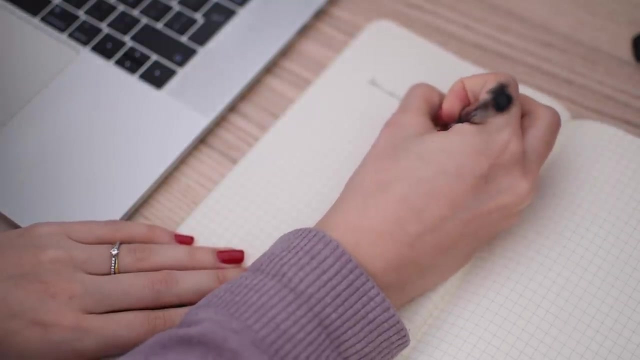 new habits, such as personal finance habits. any time of the year, January is that type of motivational month that feels perfect for this. Today, we talked a lot about budgeting and personal finance, and although anyone can learn how to do this, there are more in-depth skills that you may learn to boost your knowledge. 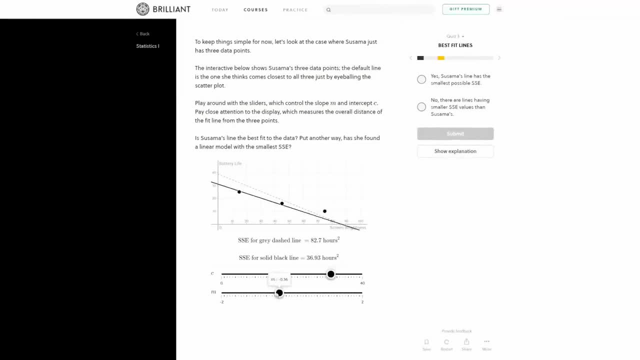 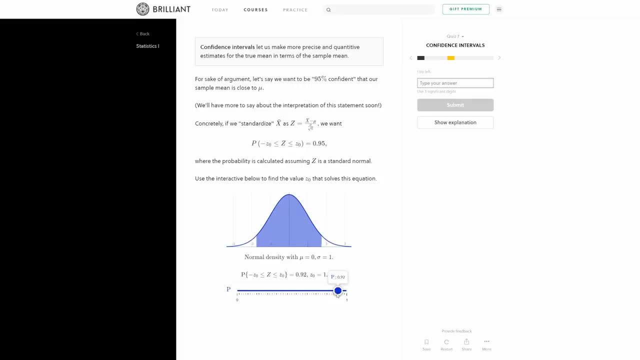 For instance, you can take this Statistics 1 course on Brilliant, which will give you hands-on experience designing experiments, and you can also learn how to build your own personal finance habits. All in all, knowing more about statistics can help you make better decisions and will. 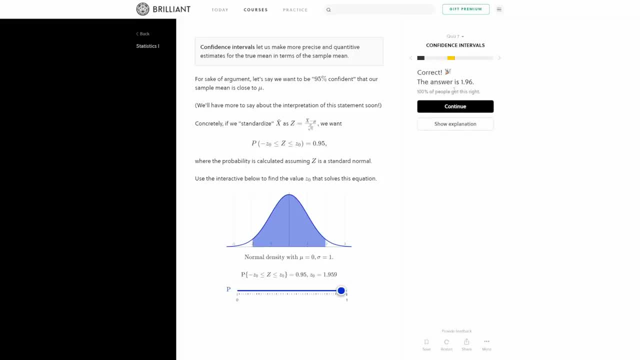 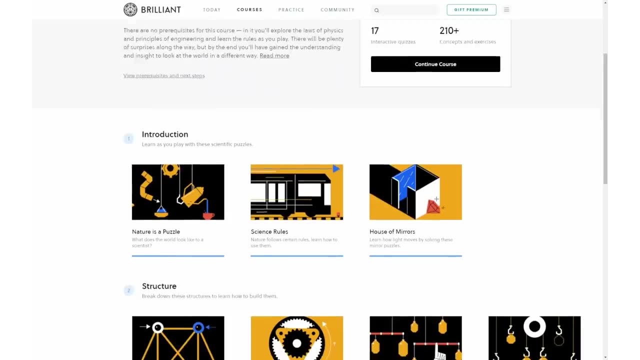 allow you to see, over time, the impact of those decisions. As I was saying, you can take this statistics course with Brilliant, which is a website and app that is free for you to try out and which makes learning interactive, accessible and fun. 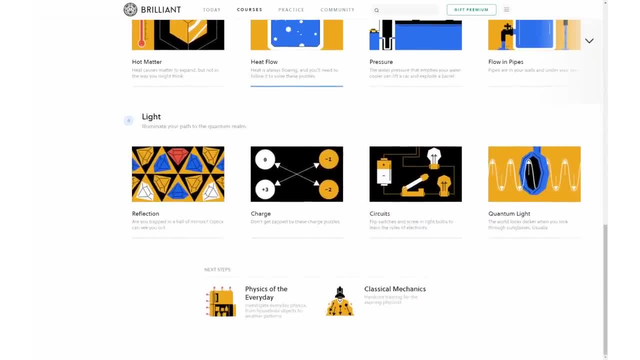 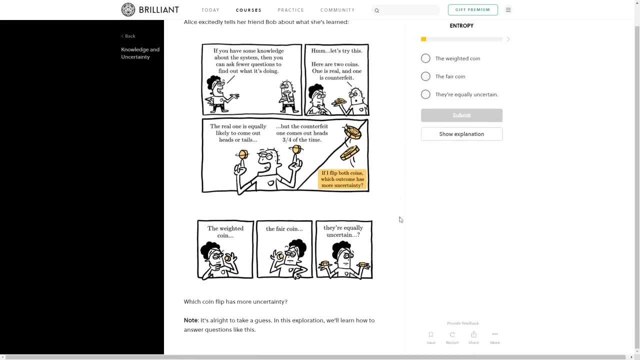 Their approach is based on problem-solving and active learning. It's about seeing concepts that you can use to solve problems. It's about learning concepts visually and interacting with them so that they stick. Their courses are laid out like a story and broken down into pieces so that you can tackle. 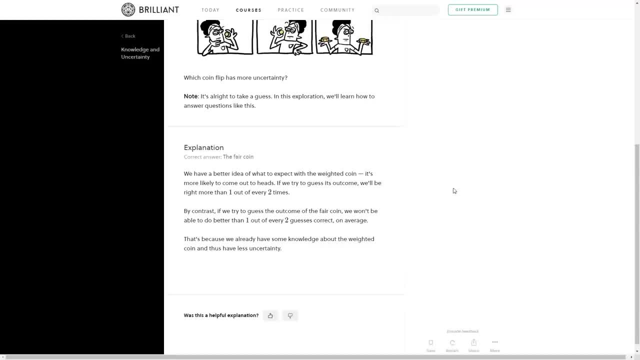 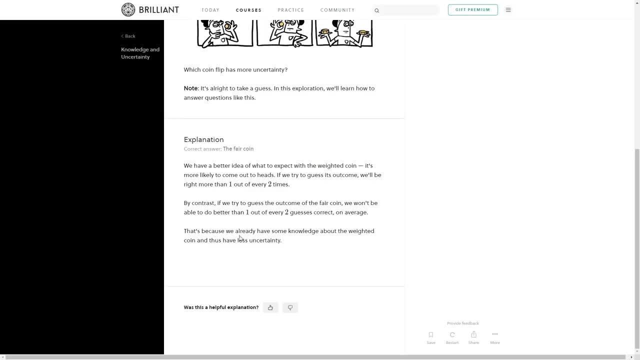 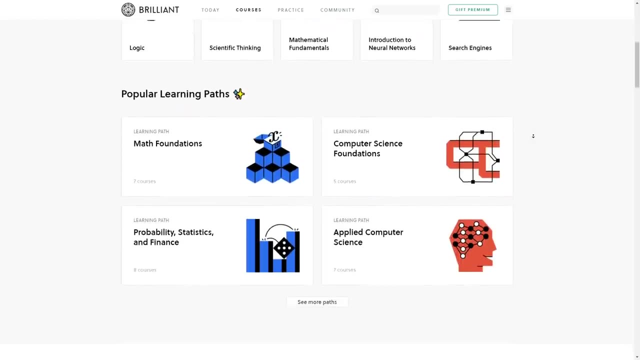 them a little bit by bit, which, as you know, is the best way to approach and successfully complete projects. Basically, Brilliant is a great platform to develop and foster a long-term commitment to learning, which is well, basically everything we promote on this channel. Just get started on your learning journey and pick a course that fits your needs. If you're interested in learning more about statistics, please subscribe to our channel and hit the bell so you don't miss a single one. See you in the next video. 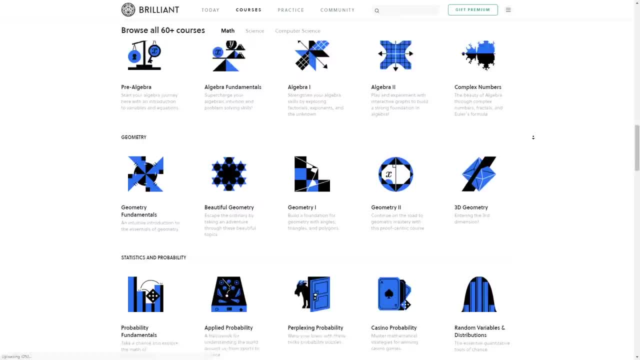 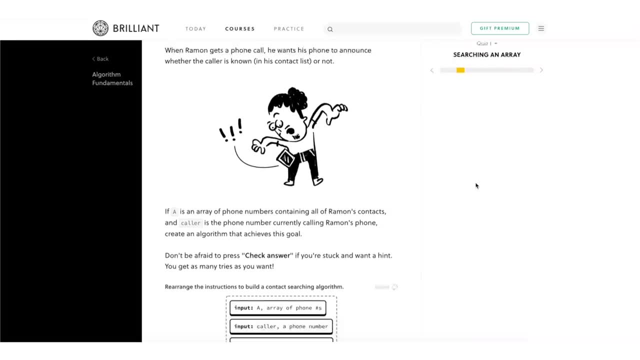 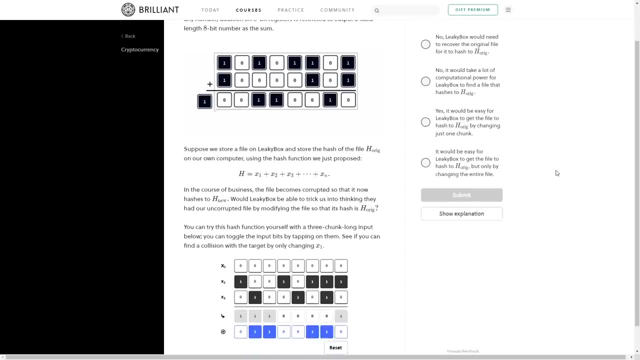 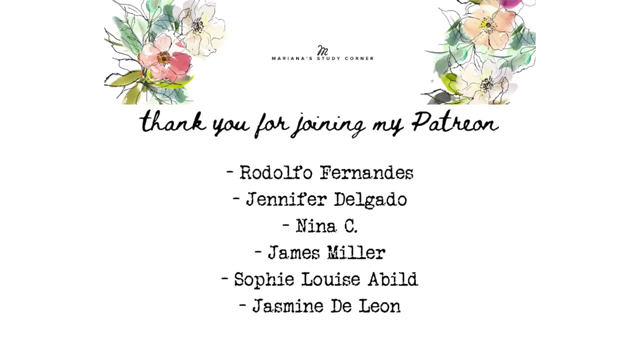 Bye. guys, Bye.